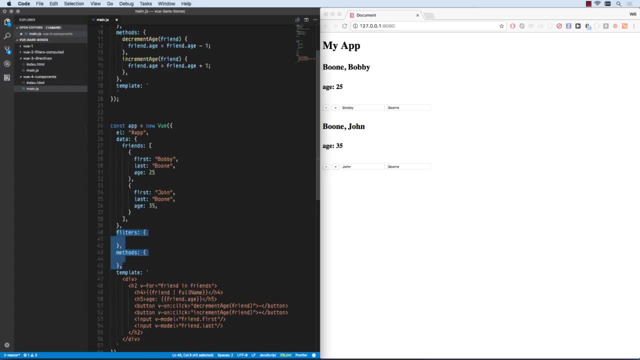 these methods there, And so actually I can completely remove those all together, And I can also remove all of this. This is stuff that has to do with a single friend, So all this information in the template here has to do with a single friend. I'm going to do a single div here. 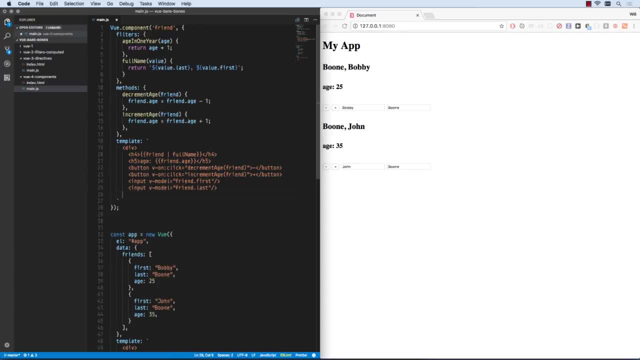 add all of that information wrapped inside of that single div. So that is our friend component. Now all we have to do is, instead of rendering an H2 for each friend, we can render a friend, And this name comes from the component name. So when we register a component by name, 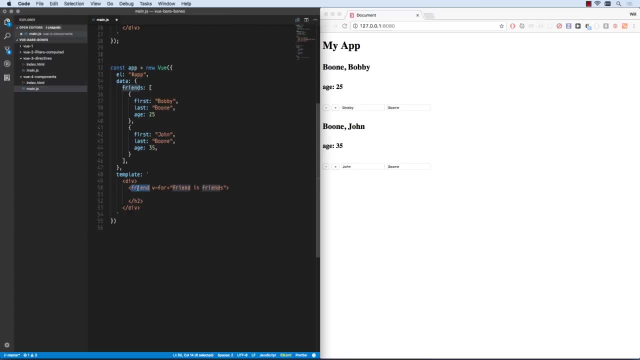 we can then spit that component out on any page as an HTML tag. So then, for each friend in our list, we are going to spit out a friend. Now this will not work, And the reason this will not work is is because it's not receiving any data. If I look here in my console, you can see: 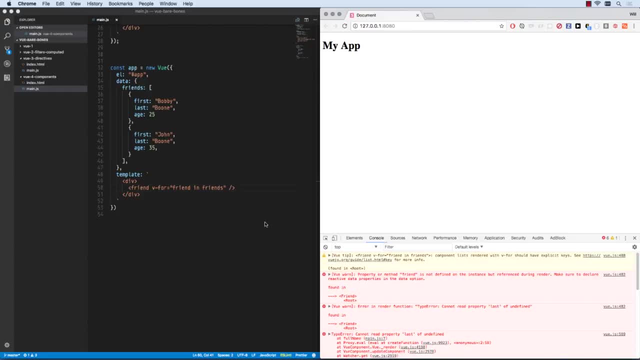 we have no property friend. nothing's defined here. So we have to say: I'm going to expect some data to be passed in here And this is called props. I'm going to get a friend object Because, as you can see, in here we're expecting friend. 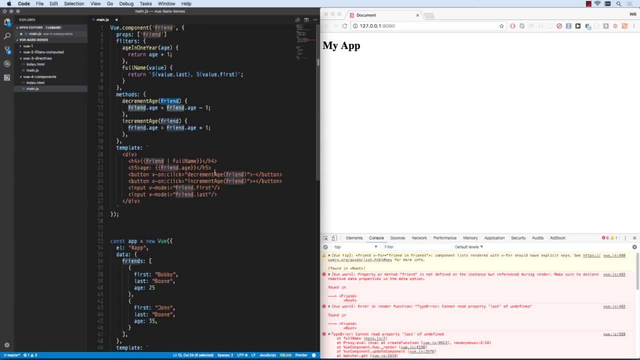 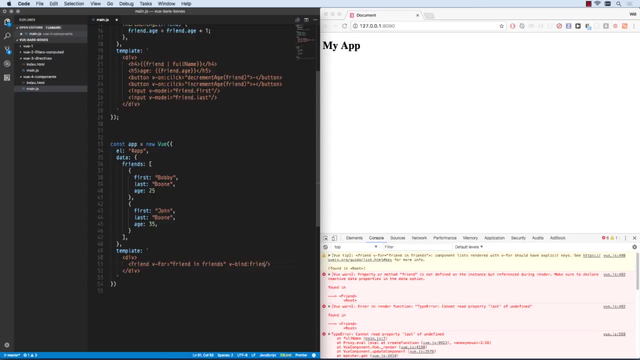 dot age friend full name. Basically we're expecting an object called friend And then we can V bind this friend and it gets the value of friend. So we're essentially saying: take this item here called friend and let's pass it in And we will call it friend in our 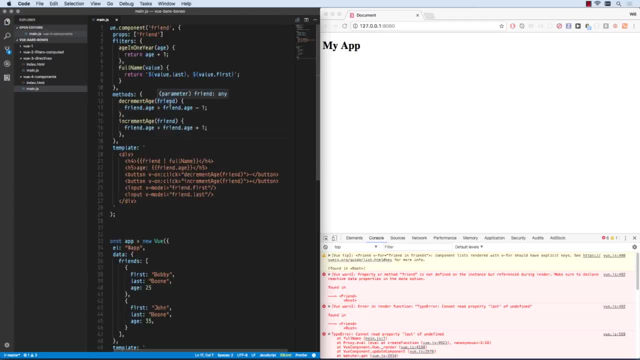 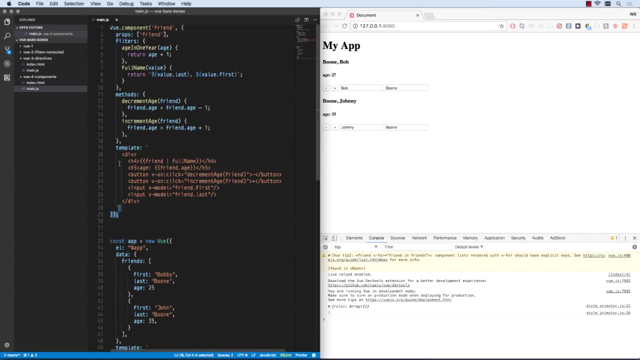 component. So there we go, that's coming in, And now everything should work. It would work if I had a comma right, Right there. There we go, You can see everything works, Everything upgrades. We can change that to Bob, change that to Johnny, And now everything's completely abstracted. This friend could be. 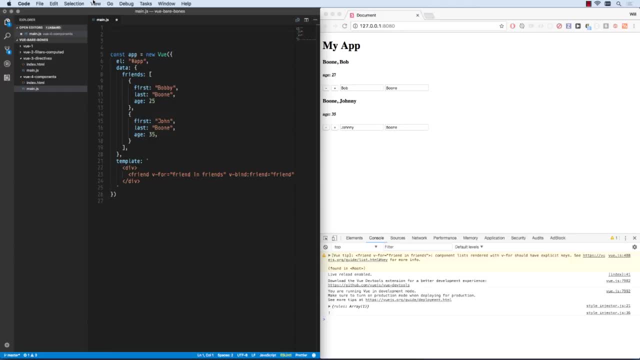 in a completely different file out there And our application would now look like this: We have our main level application with our main level data only, And then we're going to spit out child components that get the data that relates to them passed down in, And that's kind of the